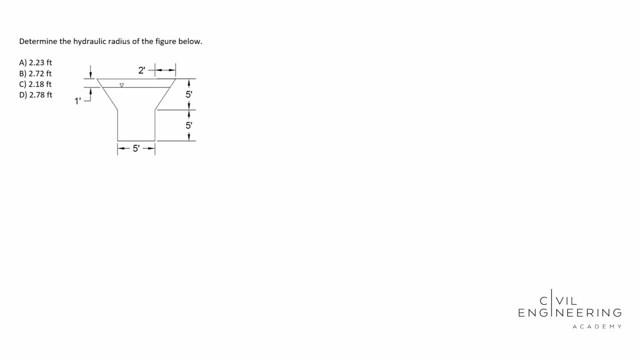 what we need in the problem- the hydraulic radius- and so if you search in your formulas for those, you're going to be finding it in the pe, on page 345, okay, and then in the fe you're going to be in 296, and so whenever you look on those you should end up with a formula that looks a little bit. 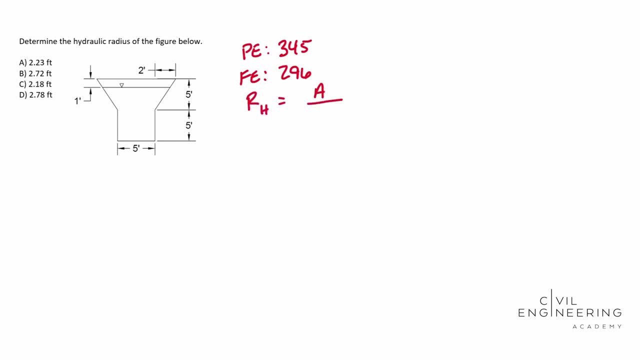 like this: the hydraulic radius is equal to your area over your wetted perimeter, and sometimes i'll throw in this w right before the p. don't be alarmed either way. it just means wetted perimeter. so we see everything that we need to solve, for we just need the area and the wetted perimeter. 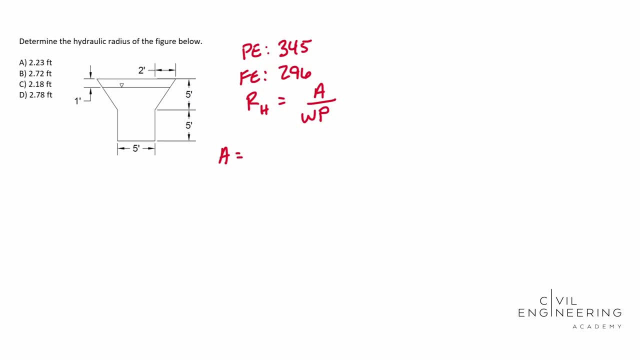 so to solve for the area first, we need to keep in mind the only thing that we're worried about right now is really the water aspect of this. the problem says that there's one foot of freeboard, so that means that it's just open air. there's no water, so we're just going to exclude that from. 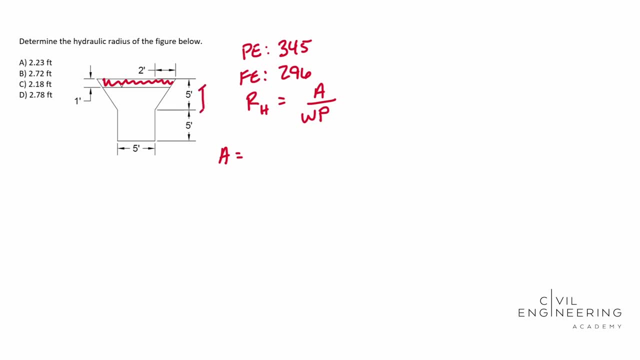 our calculations, and so we're going to use this depth here of four feet for our calculations. so, for this area, the trick to this guy is really just split it up into sections, and so we can have a rectangle here, rectangle here, triangle and triangle, and so that's what we're going to do, so zooming in real quick to these triangles. 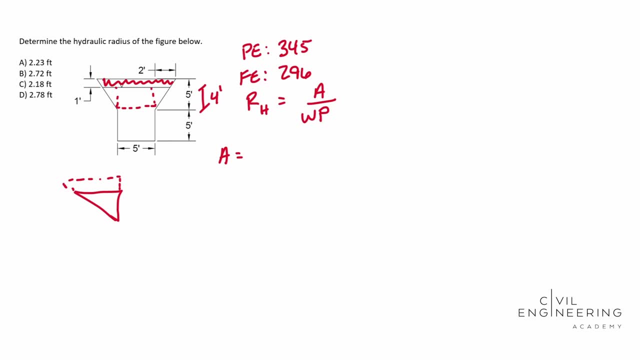 you can really mess this up in multiple ways. we see that our water level is one foot below, like i said earlier, and so the depth or the the dimension here is actually including that air space, and so we don't want to do that right, we, we don't want to include that, this guy's four feet. 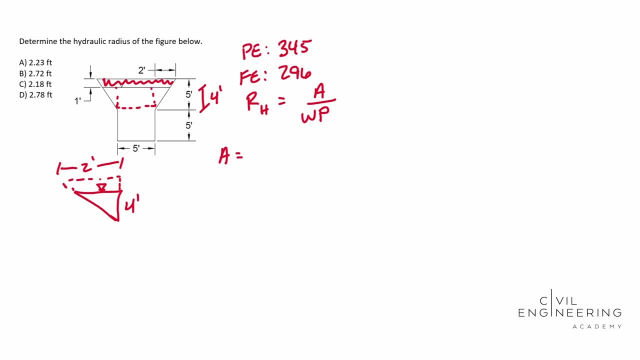 and so the way that we get by with this is: we create similar triangles. we understand this is one foot up here, so, doing that, we know that two is associated with five and that's going to be equal to something associated with four, and so what we're solving? 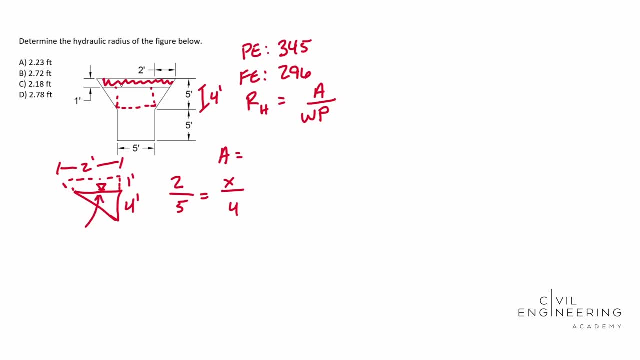 for is this dimension right there, that's. that's literally what we're solving for- is the length along that side. so whenever you do that, you end up with 1.6 feet as that dimension, and so we're going to use that in our area calculations. so, moving on here, we're going to include that first. 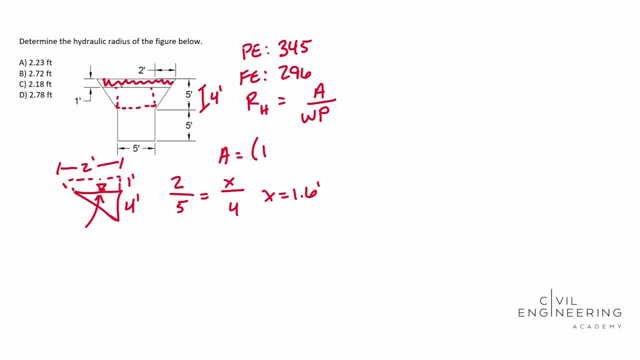 triangle base times height divided by two percent. and u to r equal two percent, or u to z, zero to ㅍr, anxious on here. we're going to include that. Then we get an inflation two. so our base is 1.6 feet, our height is four feet, and then we're going to divide that by two. 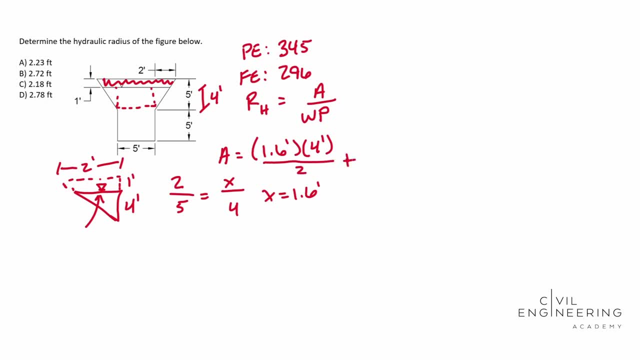 and so we're going to add our next section. now, this next section is going to be this rectangle that we created, this five by five rectangle, and so i just kind of handed towards it. the area is five feet times five feet, and then we're going to add the next rectangle. let's just work from left. 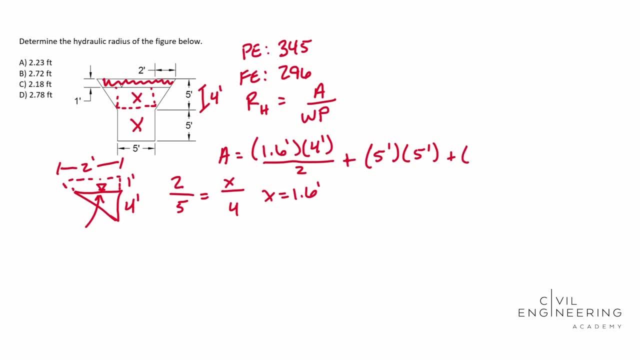 to right here. the next rectangle is four feet by five feet, so four feet times five feet. and then we have another one of those triangles that is 1.6 feet- got ahead of myself: 1.6 feet times four feet. and then we divide by two. so whenever you add all those guys up, your area should end up being 51.4. 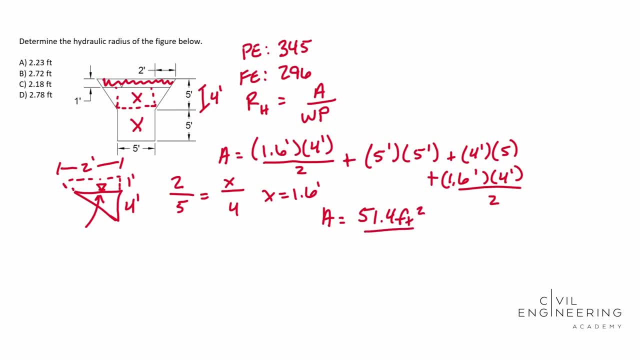 51.4, and that is square feet. okay, so we've solved for half the equation. now what? now we need to solve for the wetted perimeter, and so, to do that, we are concerned with every piece of material that is touching that water in our open channel, and so that is just this part, that's all it is. so, doing that, our p 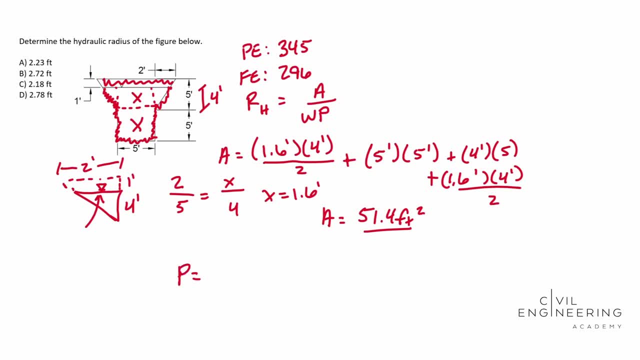 is equal to well. we need to solve for this side, we need to solve for what this hypotenuse is, and so a square plus b- predecessor squared, equals c squared. you end up with square root of 18.56, and so this is using, uh, that 1.6 feet, so 1.6 squared. i'll go ahead and do. 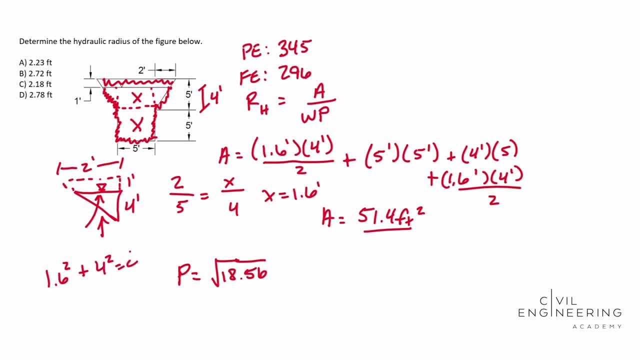 it plus your four squared equals your c squared, and so that's where that square root came from. and then we're going to add our next side, which is five feet. okay, and then we're going to add the bottom of our channel, which is five feet, other side of our channel, which is five.